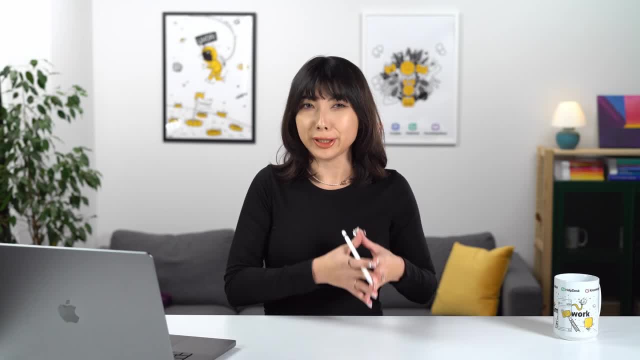 your questions and smiling. Unlike humans, who need to sleep once in a while, chatbots don't need to at all. They can also perform many additional tasks in the time a human would eat their lunch. If you have a lot of recurring questions from your customers, a chatbot can. 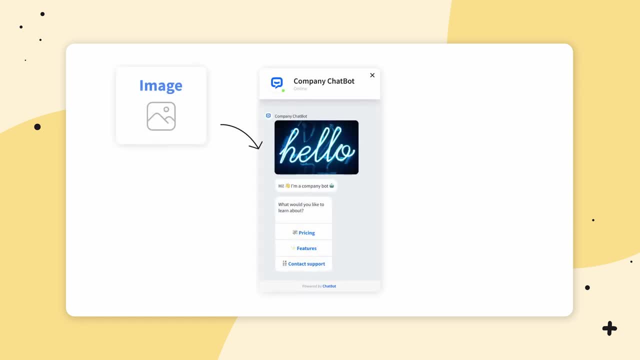 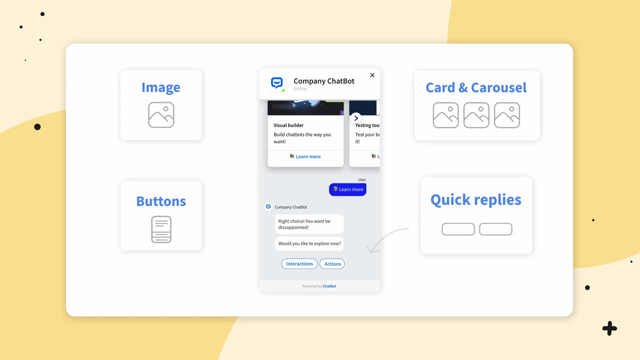 answer them quickly without burdening your support team. If you want to make it easy for your customers to sign up for newsletters, if you want to make it easy to give them coupons and discounts if they meet certain conditions, or if you want your customer support team to only handle the most complex cases, then a chatbot can do all of that for you and, at the same time, speed up your response rate and ease the burden on your team. Number two: have a dedicated customer support team If you still aren't ready to go for automated systems, because you want to provide a human touch. 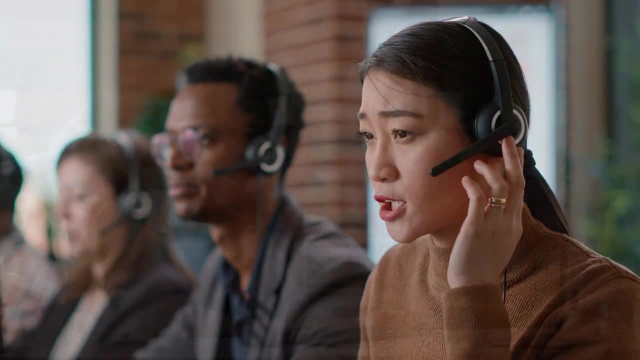 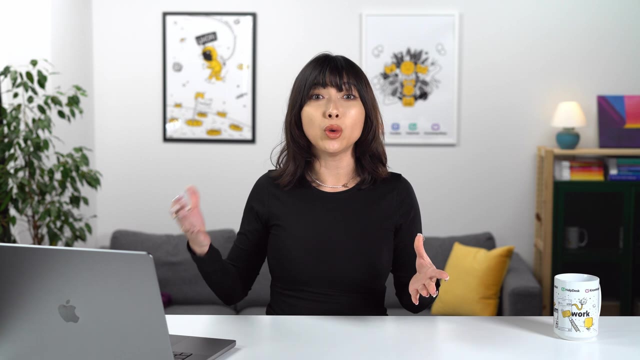 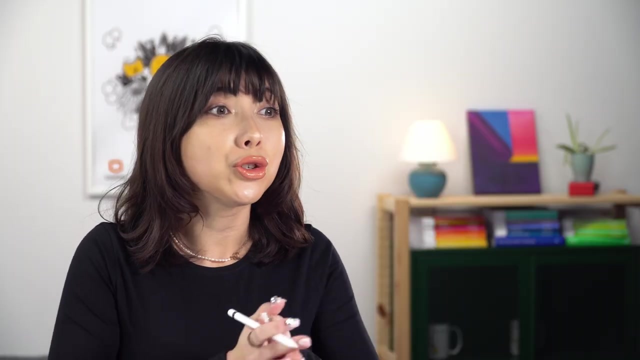 to the way you communicate with your customers, then you can have a dedicated customer support team to handle all of the inquiries. Your customer support team can help ensure that customers' questions are answered quickly via phone, email or chat. How do you do it? Or, more like, what can you do to ensure your 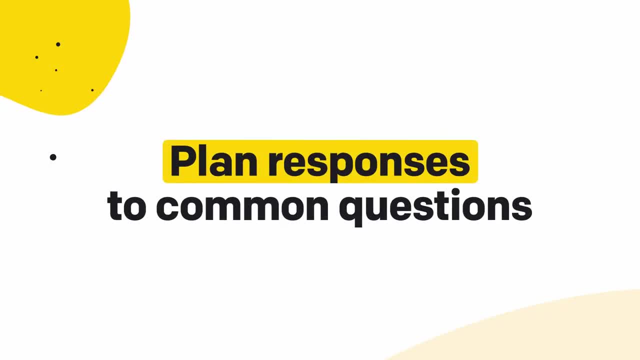 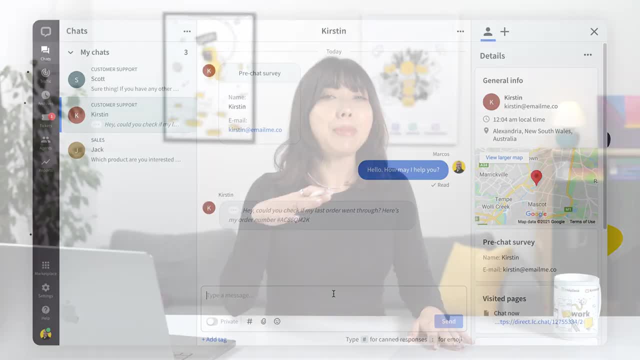 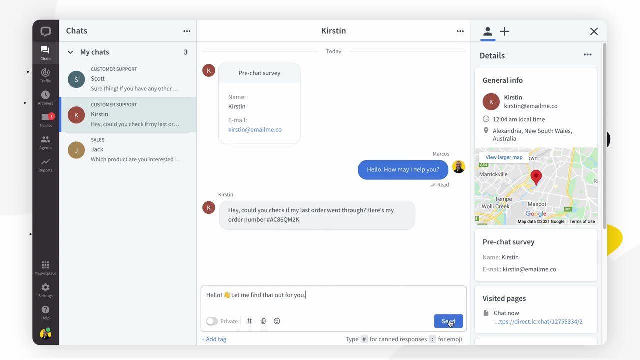 customers' questions are answered quickly. Plan responses to common questions. There's likely a small number of common questions or issues that customers are likely to have. One of the best ways to respond quickly is to have prepared responses you can send to your customers instantly, Spending the time now to make resources that can later be shared with. 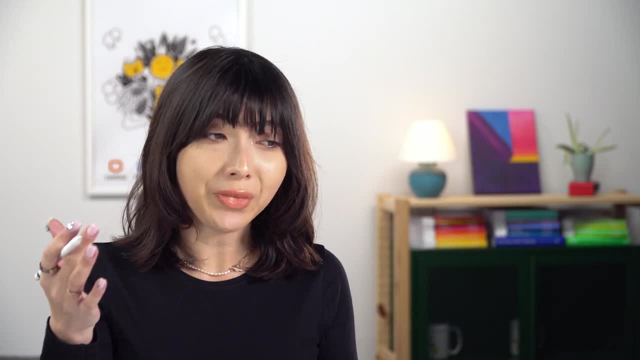 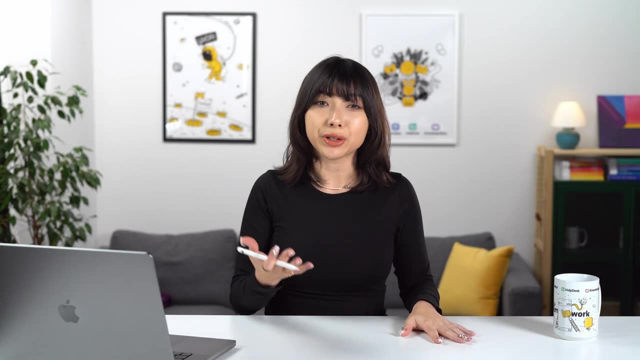 your customers will save you a lot of time down the road. You can create email and social media templates, since carefully choosing the right words and tone for your customer interactions in real time is difficult, So take the time to craft the best response and use it whenever you. 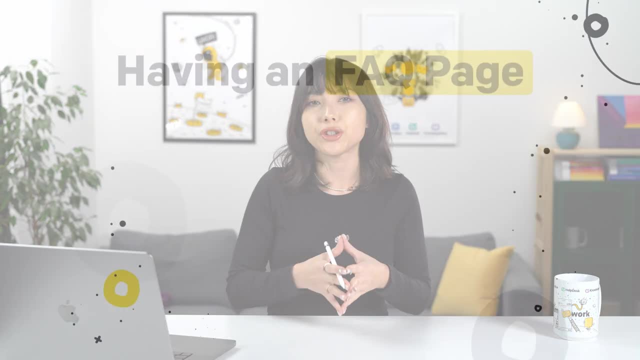 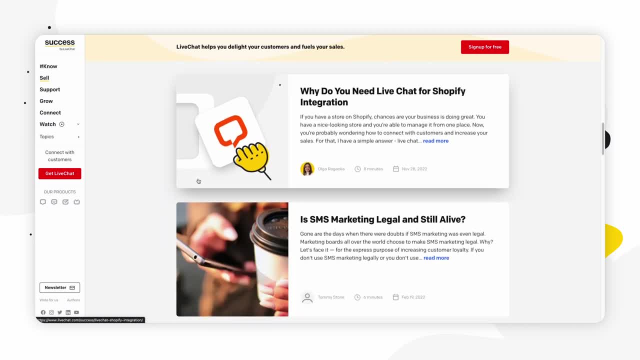 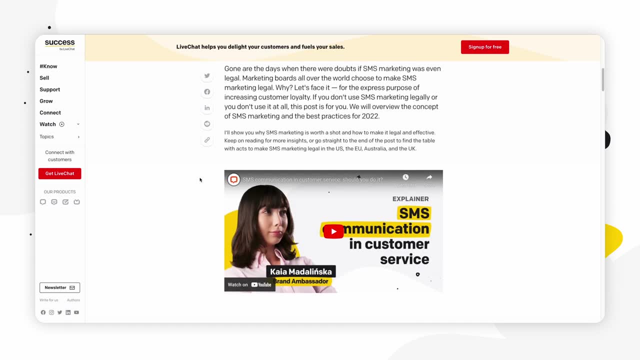 You can also make pages that explain or solve common problems people have. This way, you can direct people to your already prepared resources instead of having to once again explain something. It's all about predicting what the customer will want to know and providing it. 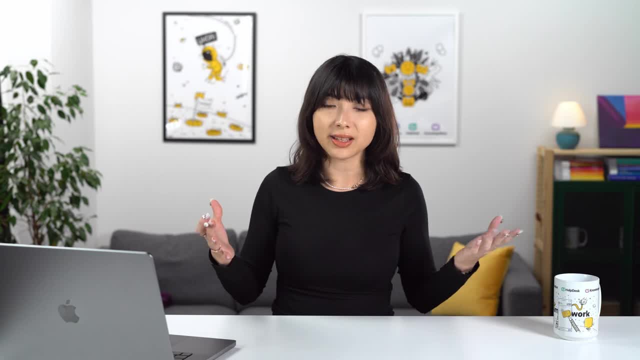 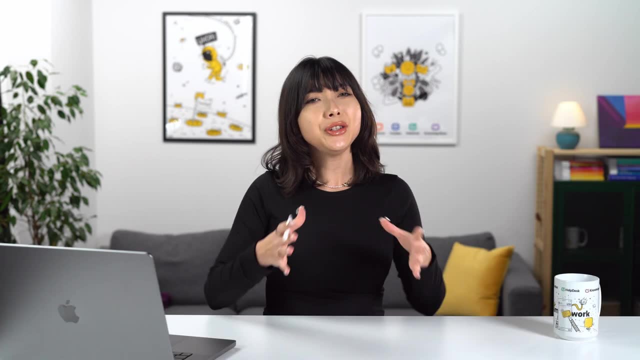 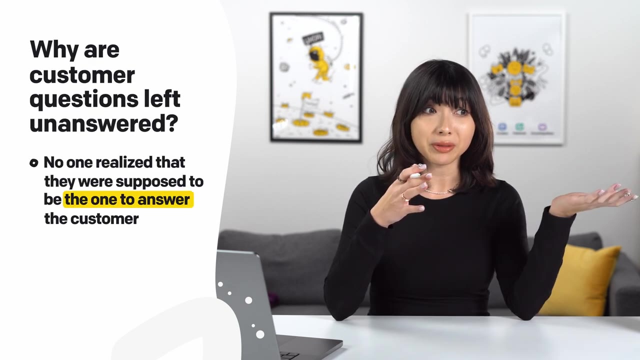 either as quickly as possible or before they even have to ask, And this way you can focus on the more difficult conversations and tasks. Set a clear notification system. There are two issues for why customer questions are left unanswered. Number one: no one realized that they were supposed to be the one to answer the customer. 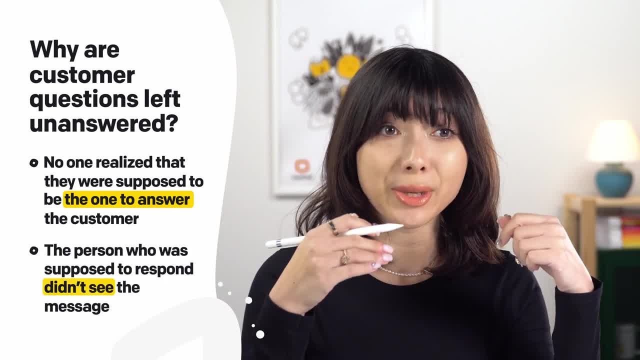 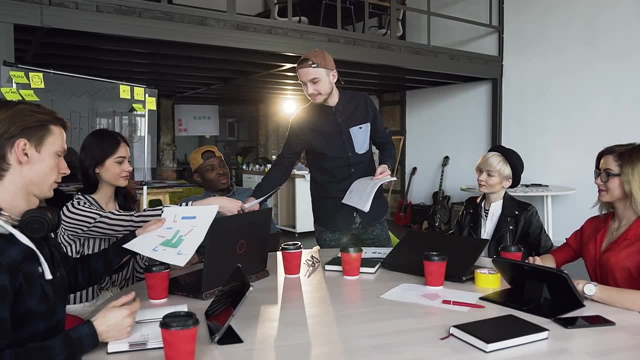 Number two: the person who was supposed to respond didn't see the message. The first issue can be easily resolved by being transparent with your team on who needs to do what and how often. Clear expectations are essential for avoiding confusion. Make sure that each communication. 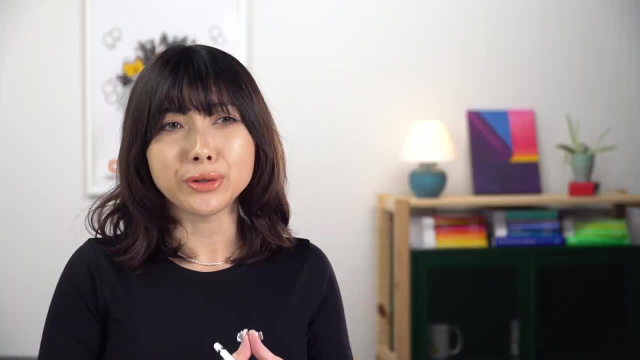 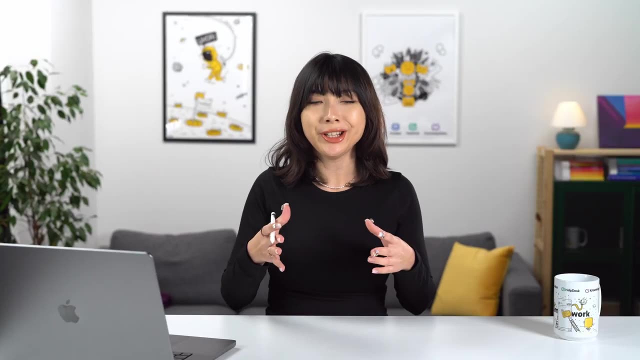 channel has a team member signed to it. Also, have a backup person who knows how to take over whenever the initial team member is unavailable. As for the person who was supposed to respond but didn't see the message, well, you need to get your team organized. There are various tools that can help you with that. 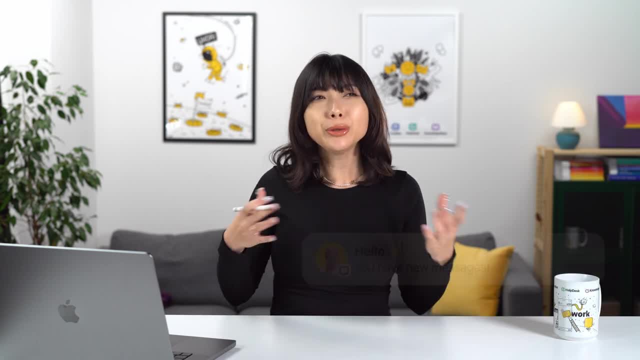 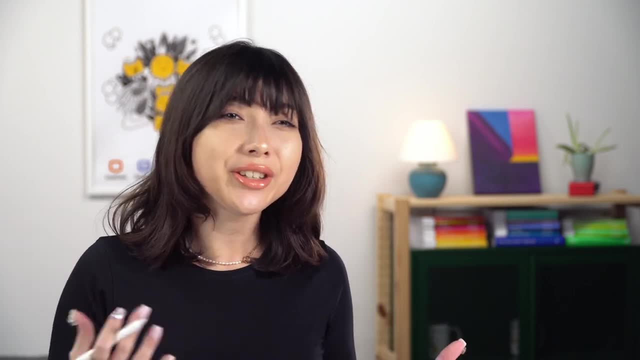 by notifying you each time a customer asks a question. Tools like Slack can be integrated with Notify to make sure you receive the notifications. Your customer service team will be alerted instantly to any mentions. This way, there won't be any more mix-ups. 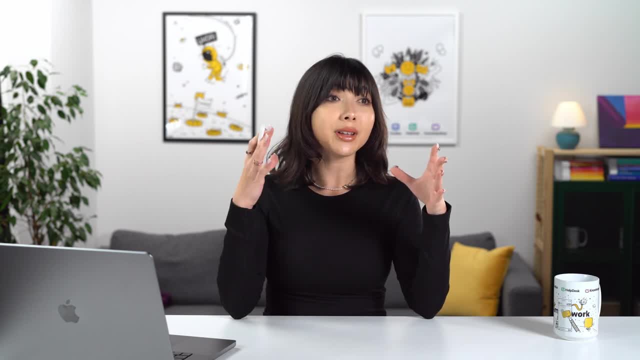 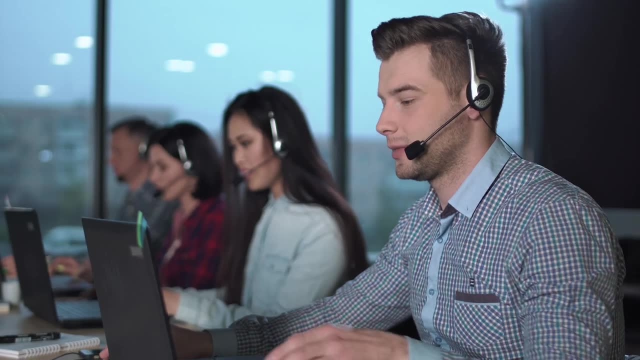 or you simply need to make sure you have a system in place that will assign the case to another team member if the first team member didn't respond. Lastly, please remember that your customer service team will always be on the lookout for any questions you may have, If the first team member 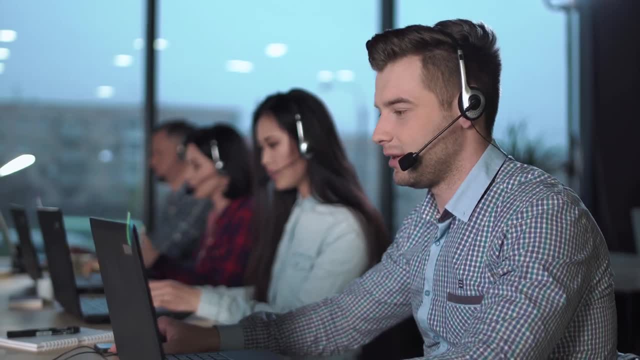 is not on the lookout for any questions you may have. you may want to make sure that they are on the lookout for any questions you may have. Therefore, it's not really surprising that there's a lot of training involved and that there are many key skills to look for when hiring your 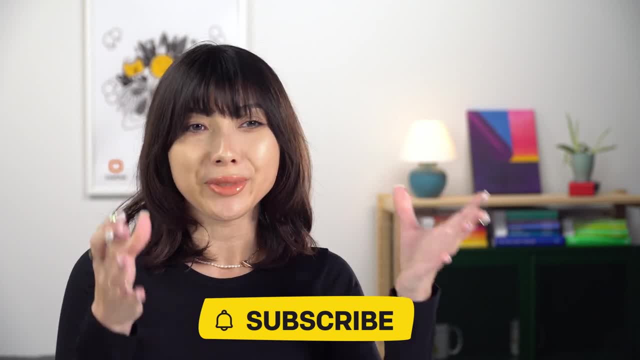 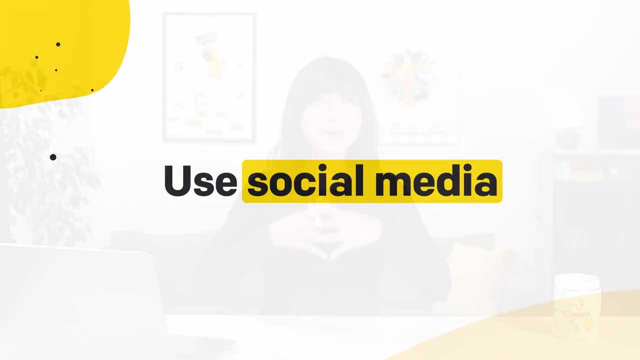 customer service team. We will actually have a video on that topic coming soon, so make sure to subscribe so you're notified when the video comes out. 3. Use Social Media. Social media platforms such as LinkedIn, Facebook, Twitter and Instagram can be. 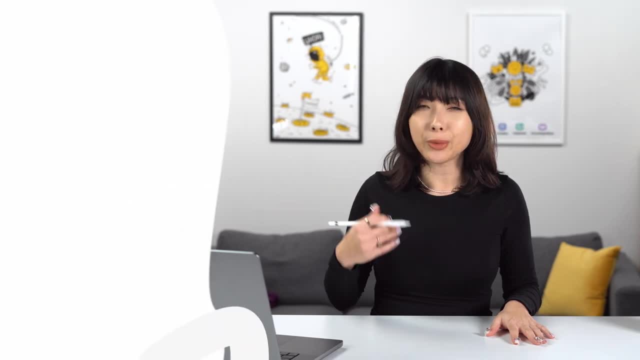 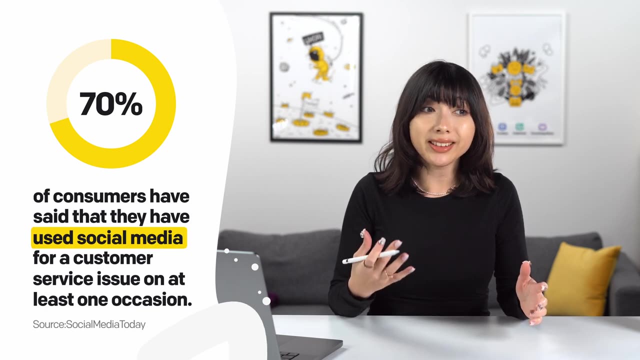 great channels for answering customer questions and providing support in real-time. Nearly 70% of consumers have said that they've used social media for a customer service issue at least on one occasion, And that's why a lot of companies provide social media customer service: because